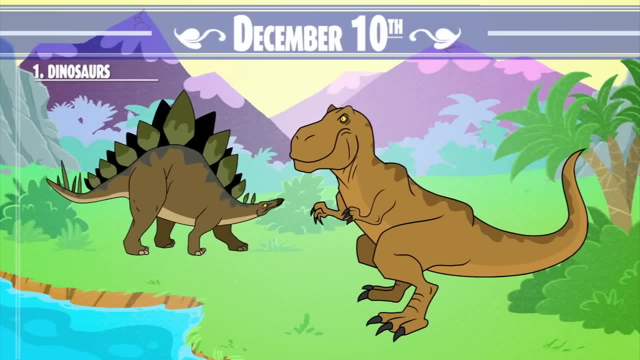 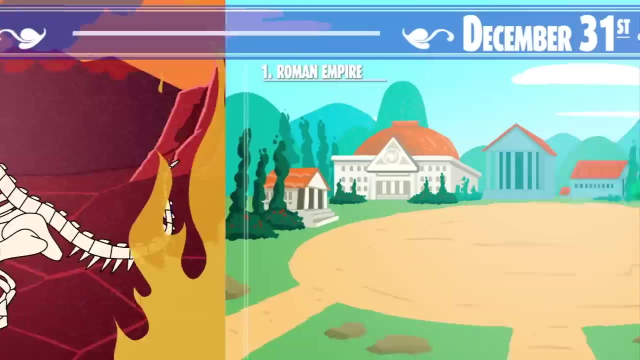 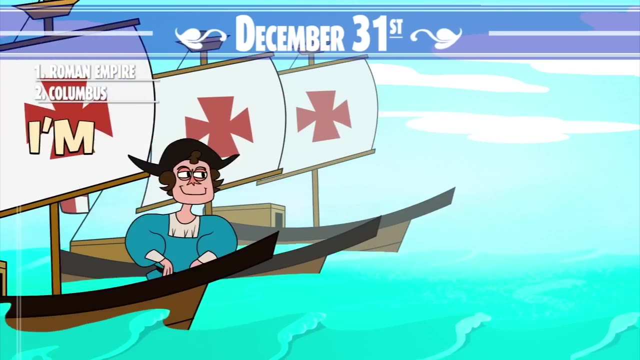 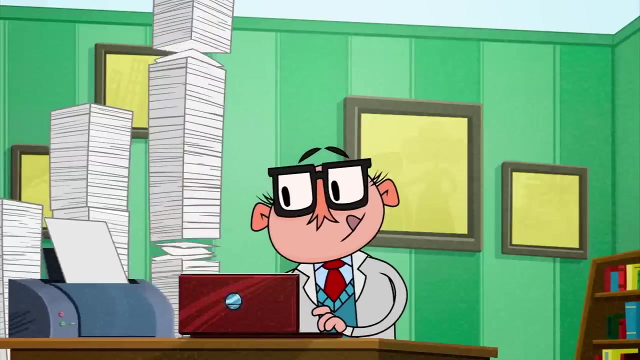 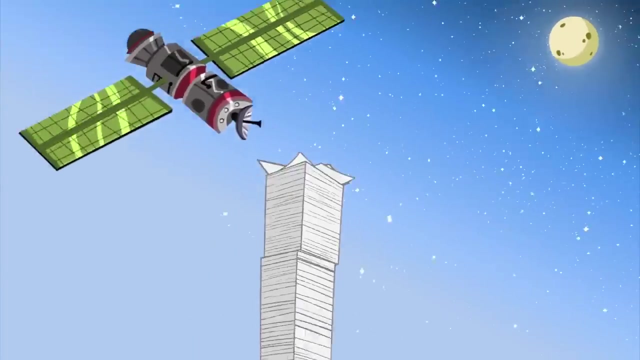 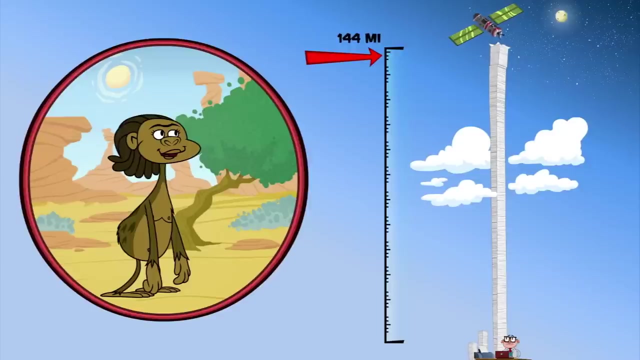 On December 10th at 1.26pm, the dinosaurs first evolve, but are wiped out by an asteroid just two weeks later. On December 31st, the mighty Roman Empire rises and falls in just under four seconds, and Columbus sets sail for what he thinks is India at three seconds to midnight. If you tried to write the history of the Earth using just one page per year, your book would be 145 miles thick, more than half the distance to the International Space Station. The story of the 3.2-million-year-old australopithecine fossil known as Lucy would be found on the 144th mile, just over 500 feet from the end of the book. 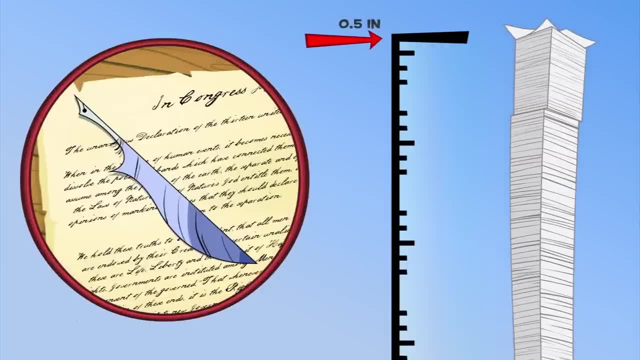 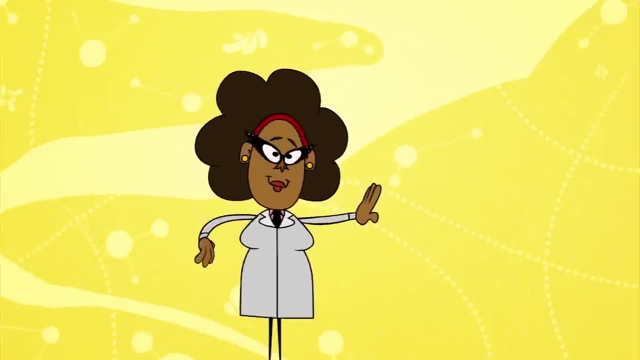 The United States of America's Declaration of Independence would be signed in the last half inch. Or if we compare geologic time to a woman stretching her arms to a span of six feet, the simple act of filing her nails would wipe away all of recorded human history. 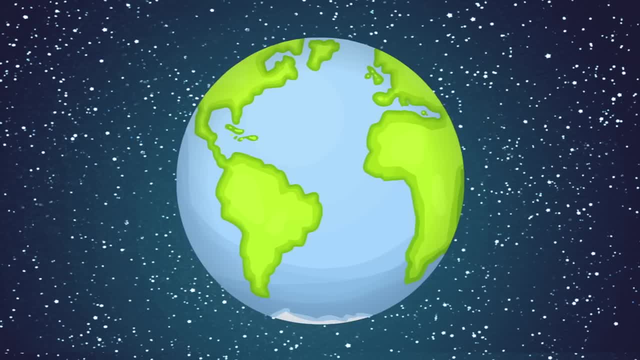 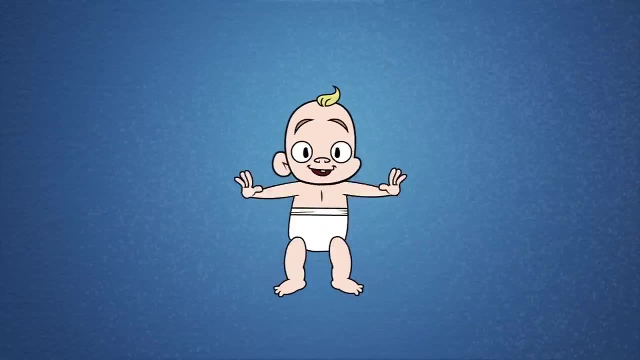 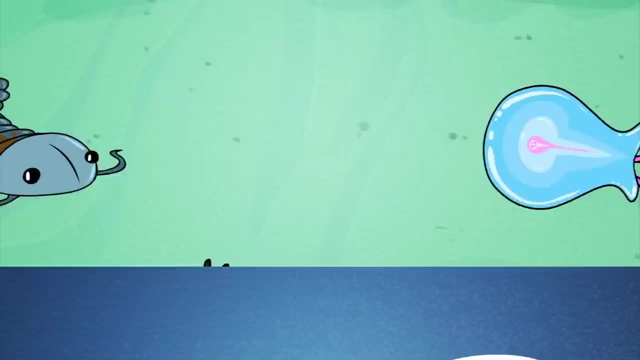 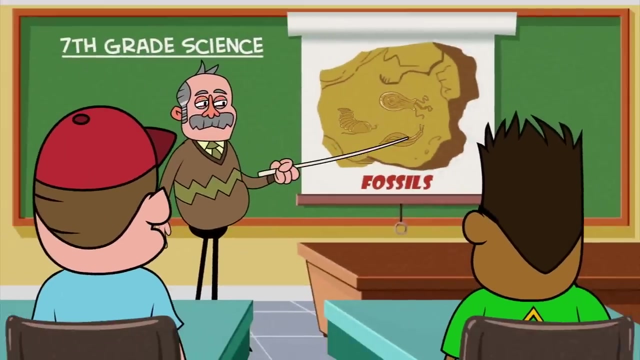 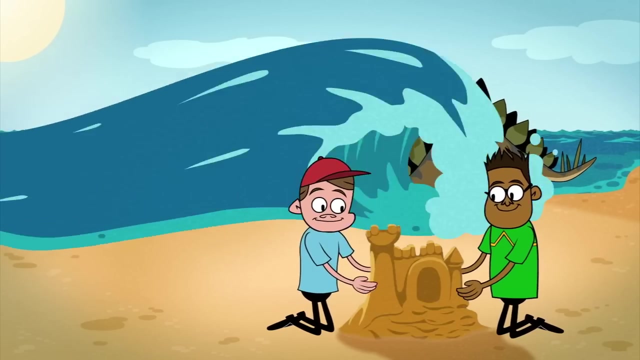 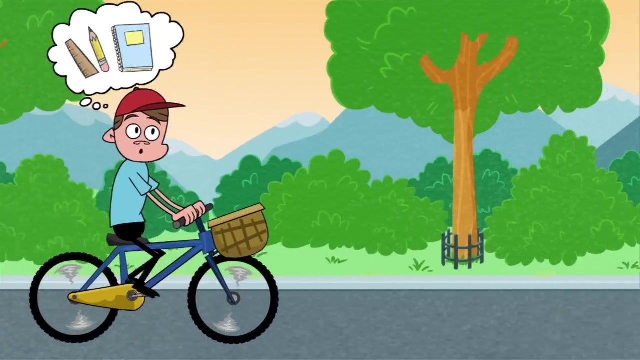 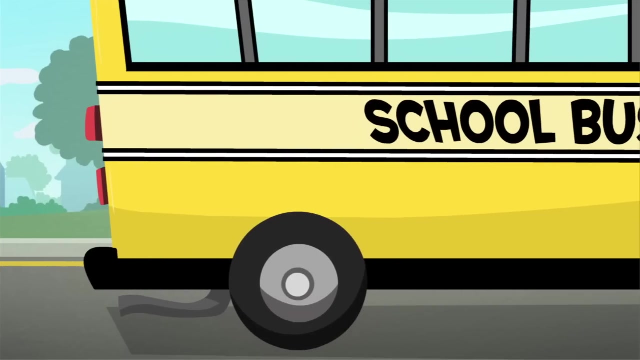 Finally, let's imagine the history of the Earth in just a few minutes. We're going to look at the history of the Earth as your life from the moment you're born to your first day of high school. Your first word, first time sitting up, and first time walking would all take place while life on Earth was comprised of single-celled organisms. In fact, the first multicellular organism wouldn't evolve until you were 12 years old and starting seventh grade, right around the time your science teacher is telling the class how fossils are formed. The dinosaurs don't appear until three months into eighth grade, and are soon wiped out right around spring break. Three days before ninth grade begins, when you realize summer is over and you need new school supplies, Lucy, the Australopithecine, is walking around Africa. As you finish breakfast and head outside to catch your bus 44 minutes before school, the Neanderthals are going extinct throughout Europe.